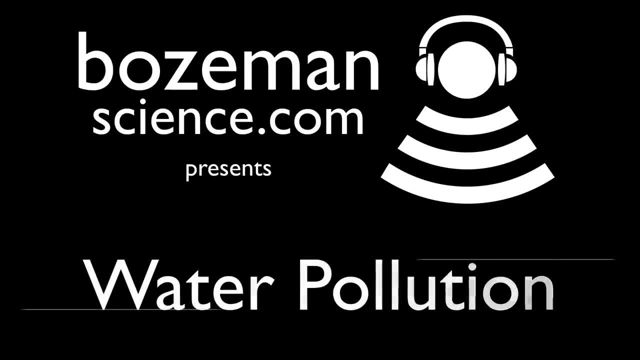 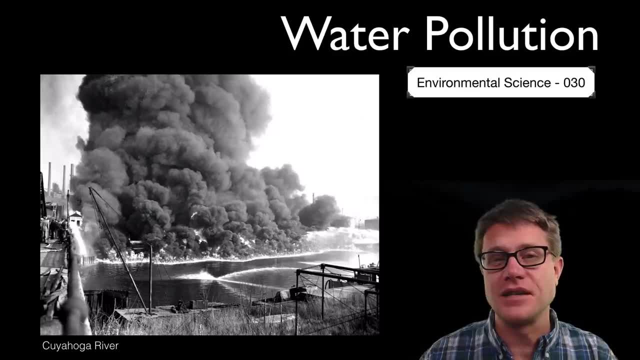 Hi, It's Mr Andersen and this is AP Environmental Science. Video 30 is on water pollution. Water pollution made headlines in 1969 when the Cuyahoga River in Ohio started on fire. This is not that fire. This is a picture of an earlier fire. In fact, the Cuyahoga. 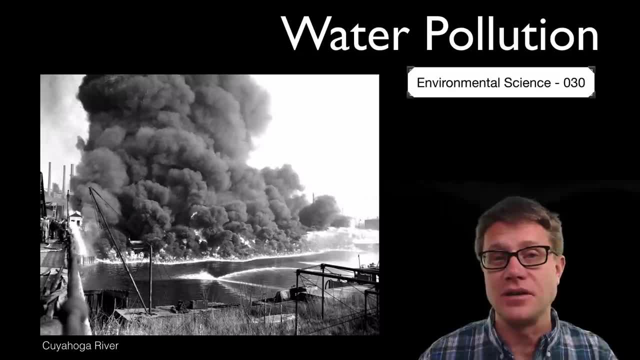 River had started on fire many times, going way back into the 1800's, But this caught people's attention, The idea that water could catch fire. It was not the water itself that was burning, But led to regulation to clean up water, And this is the Cuyahoga River today. 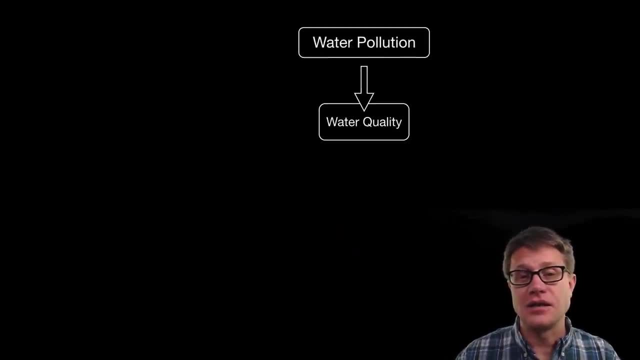 It's cleaned up. The job is not done yet. But water pollution is anything that decreases the water quality of lakes, streams, rivers, things like that, And so we categorize water pollution depending on where the pollutants are coming from. Point pollution would be. 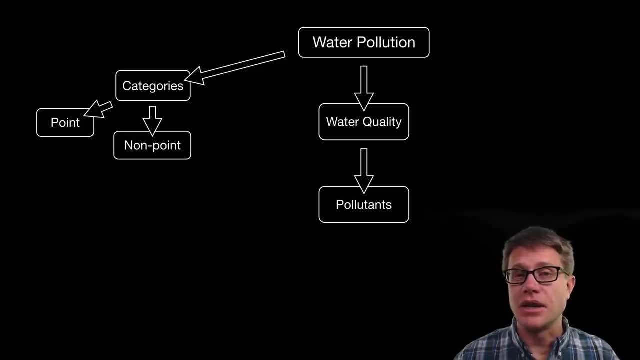 coming out of one pipe or one ship, for example, We can have non-point That is coming from, for example, all of the farmer's field in an area, And then we can have ground water pollution. So it is in that water table, underneath the ground itself, The major pollutant is going. 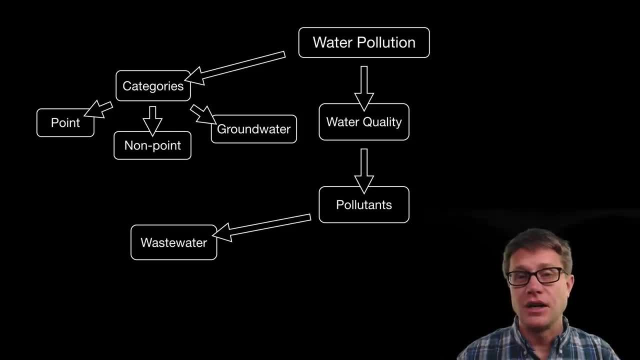 to be waste water. This is animal and human waste, And so that waste has to be broken down, And we generally do that using bacteria, And as the bacteria break down the waste, they require oxygen to do that, And we can measure how polluted that waste water is by looking. 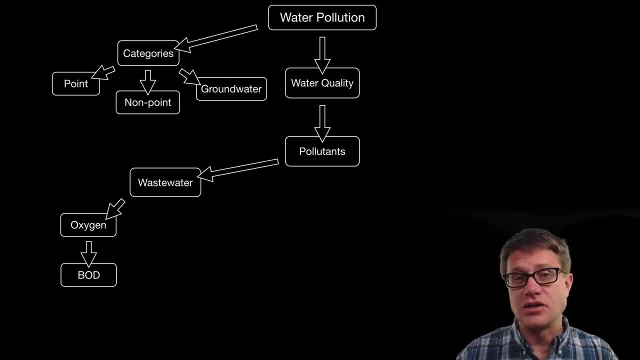 at what is called the biochemical oxygen demand. How much oxygen are these bacteria requiring? Now, as they do this, they pull oxygen out of these surrounding material and can lead to dead zones. We see this along a lot of the coasts in the US. We also get an increase in nutrients in that area, And so you will get eutrophication. 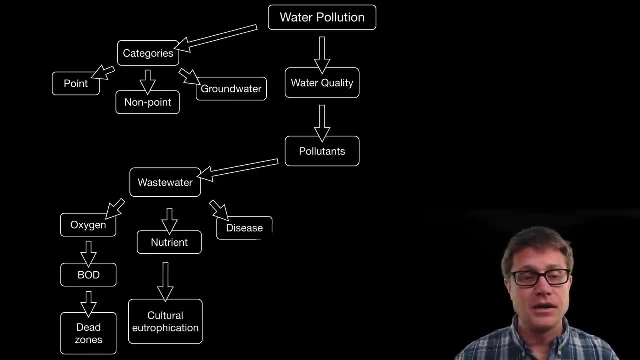 So we get a bloom of algae producers in that area, And then also waste water carries disease from one area to another. Cholera is a great example of that. It is not only waste water that can lead to pollution. We can also have chemicals like metals, acids, synthetic material. 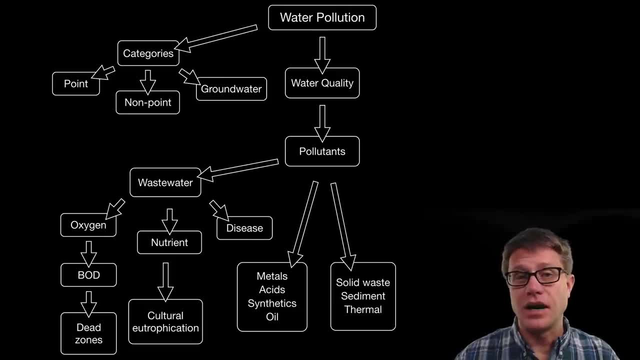 like pesticides and oil. And then we have nonchemical- Not at the molecule level. So an example could be garbage that is found, A sediment that is found, Or even heat can lead to water pollution, And so we have cleaned that up. We have the Clean Water Act, We have 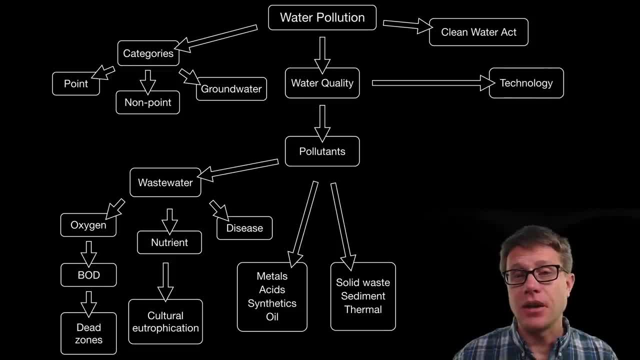 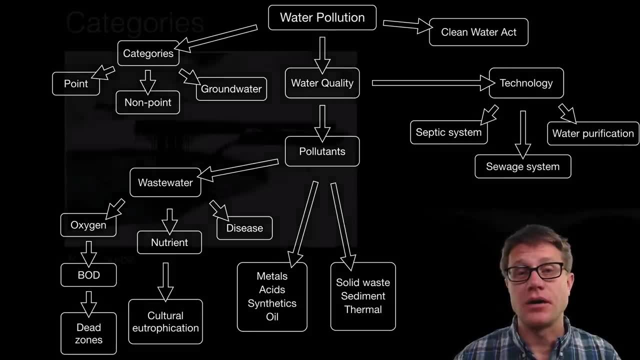 the Safe Drinking Water Act as well. And so how do we clean up that water? through technology, So we could use a septic system, A municipal sewage system, And then we can treat our water as well. And so the categories of water pollution we can have: point pollution. This is an example. 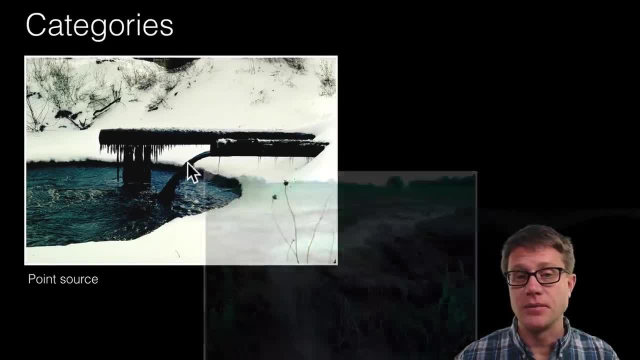 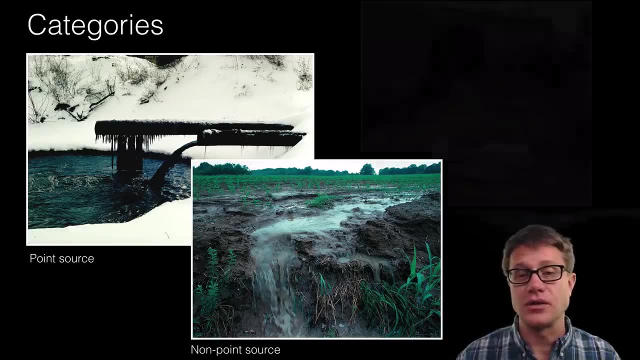 of that. We have got sewer coming right out of a pipe into a river. We can have non-point source. This could be all the water washing over farmers fields, pulling pesticides and nutrients into the water supply, And then we can have groundwater pollution. So in this, 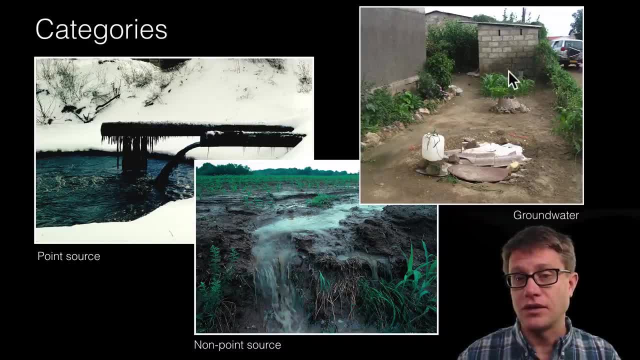 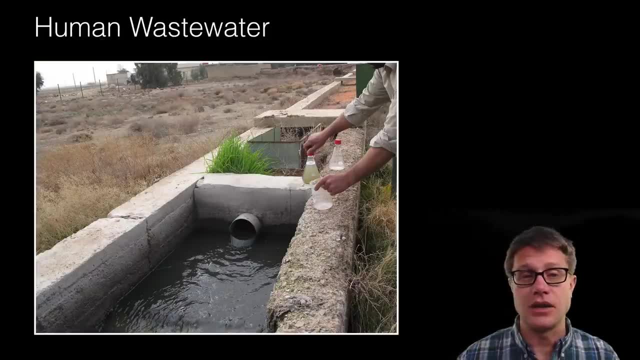 case. we have got a latrine over here, And so the human waste is going to move down underneath the ground into the water, And you can see, their well is right here, So you can get contamination like that, And so the major pollutant is human waste water or sewage, And so this person 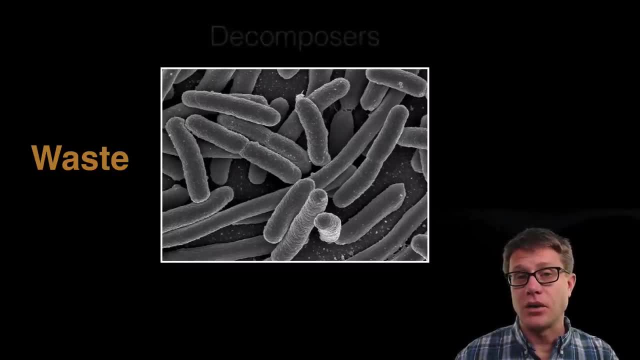 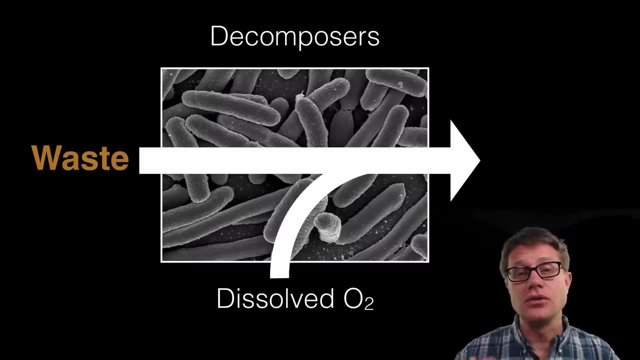 is testing the water here. What happens is that waste is broken down by bacteria decomposing- bacteria like E coli. But to break it down, they require dissolved oxygen, Just like you do as you breathe, And so we can look at the amount of oxygen that is being consumed. 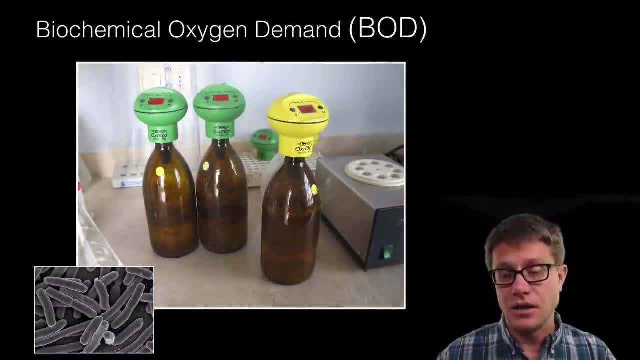 and that tells us how much waste there is. And so we use a standard called the biochemical oxygen demand. What you do is you measure how much oxygen is being produced by these decomposers. Our standard is how many milligrams of oxygen- dissolved oxygen- per liter is. 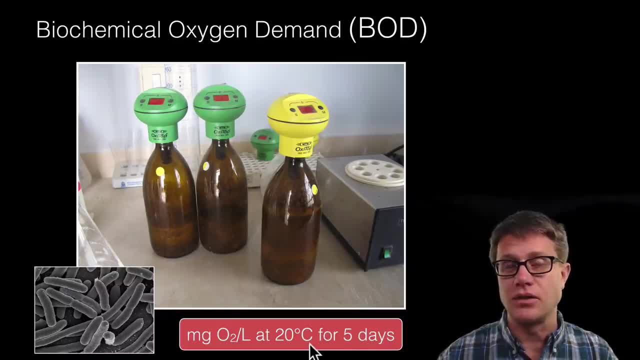 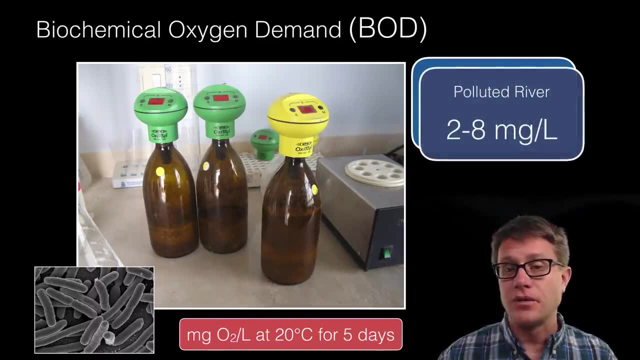 used over five days at around room temperature or 20 degrees Celsius. And so if we were to take a pristine river, its BOD is going to be less than one milligram per liter, But if we are looking at a polluted river, it is going to be a much higher amount. If we look 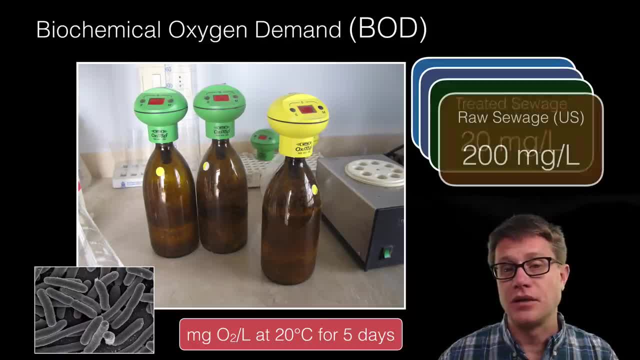 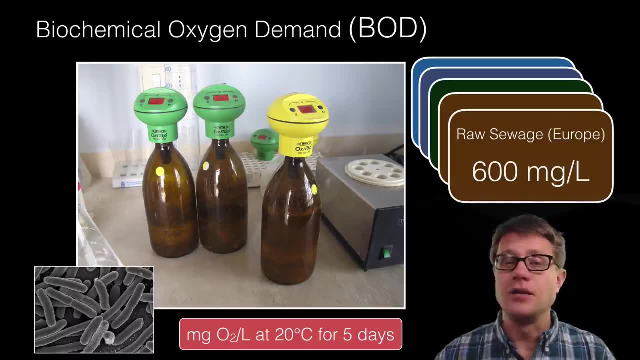 at sewage- treated sewage- it is going to be 20 milligrams per liter. But if we look at raw sewage in the US it is around 200. And if we look at it in Europe it is going to be around 600.. Now you may think: why do they have more polluted sewage? It does not. 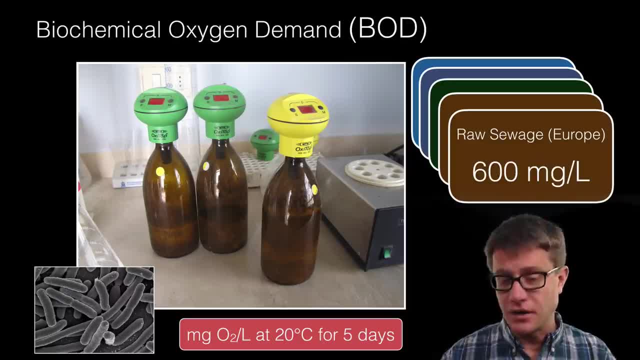 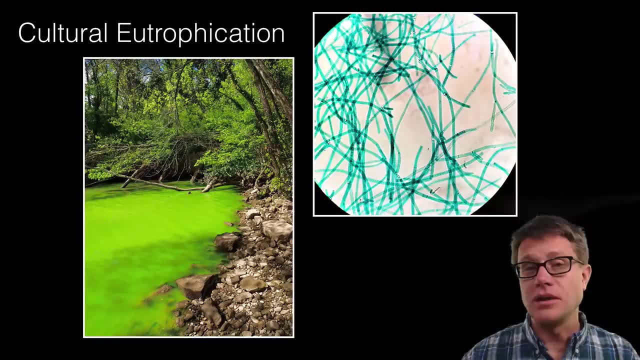 have anything to do with the waste. It is that in the US we produce so much water, We take so many long showers, We flush the toilet, And so as we go through the year we are going so as we do that we are diluting these BOD numbers. Now it also leads to increases in 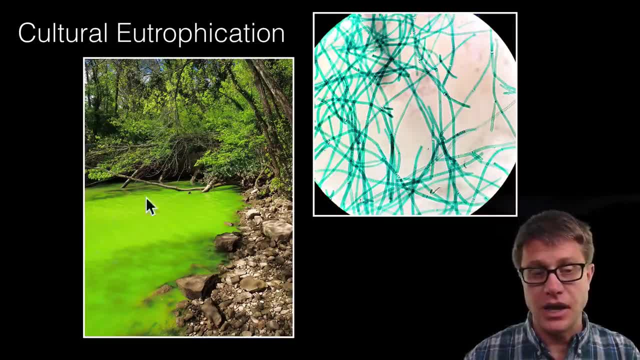 nutrients and eutrophication. So this is pollution leading to an algae bloom. We have a bunch of blue, green algae that are using the nutrients in it, And so you get a huge explosion of growth. You might think this is a good thing, But what happens? this is an algae bloom off. 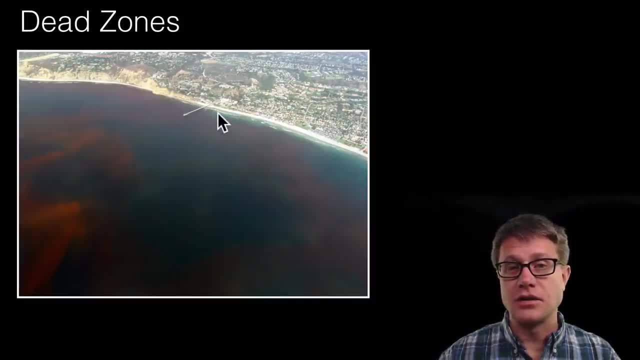 the coast of California, And so as you get an algae bloom like this, there is a bunch of producers algae in that area, But then they eventually die, And as they die, these same decomposers are going to break it down And as they do that, they pull oxygen out of the water, And so we are producing what are called 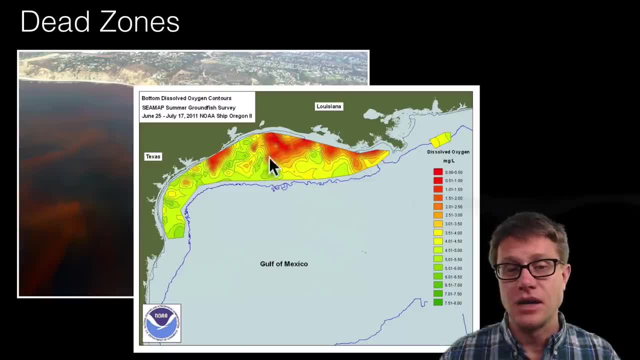 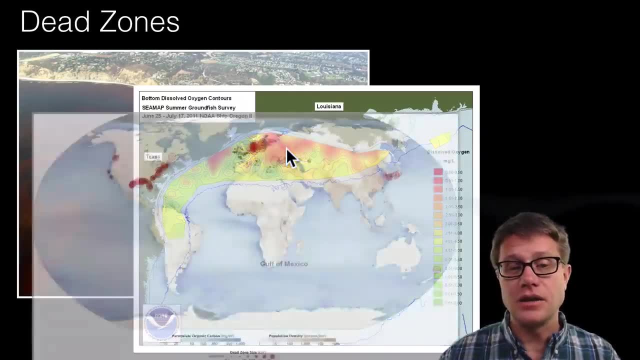 dead zones. This is a massive dead zone around the size of Rhode Island in the Gulf of Mexico, And what we are doing is pulling the oxygen out of the water, And so fish are dying, Shellfish are dying, And you can see that we have dead zones all around our planet, But it is going. 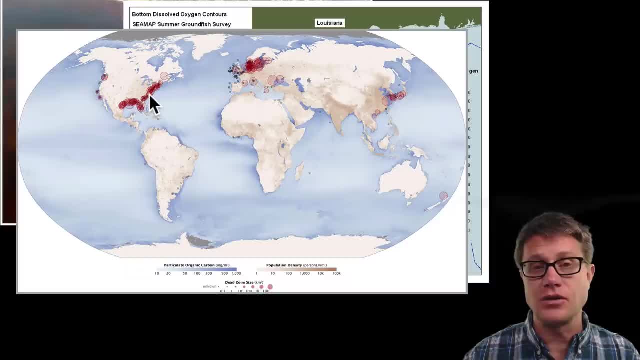 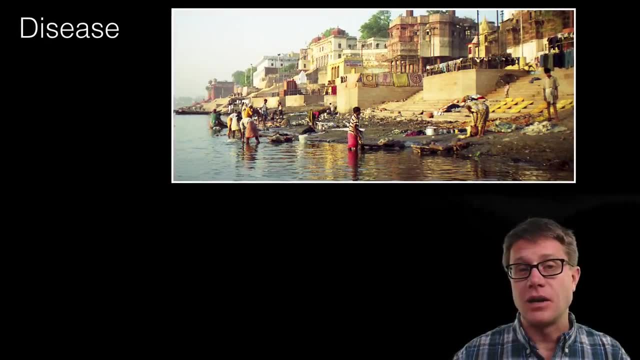 to be aggregated in areas where the water is moving out into the ocean with huge amounts of nutrients. So we have this eutrophication and then these dead zones are being created. Also in that polluted water. we have diseases, We have diseases, We have diseases, We have. 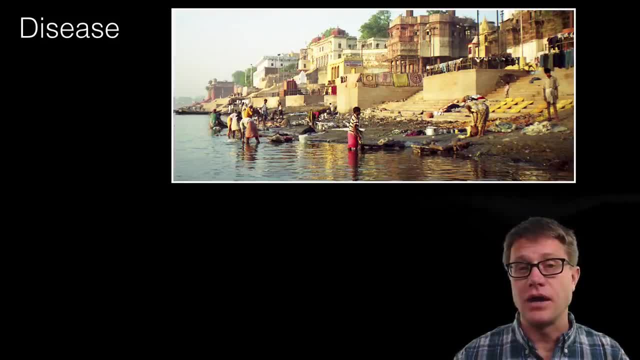 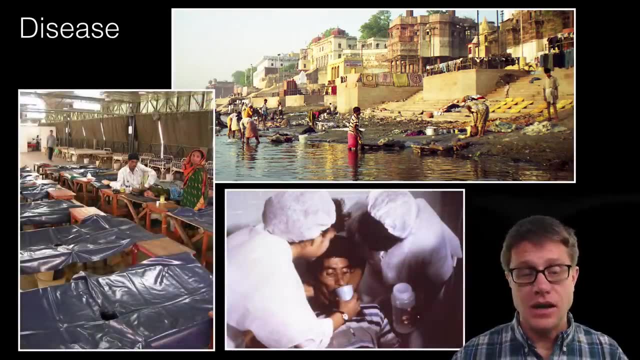 disease, And so in India you can see here that they are washing themselves in the water. But we also have wastewater in there as well, And sometimes we are pulling the drinking water out of there And so it can lead to disease, Cholera outbreaks in India or in. 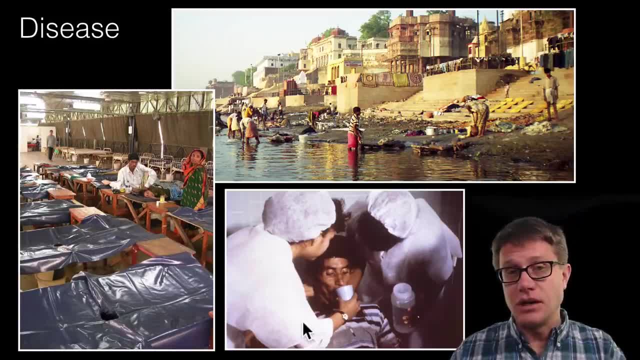 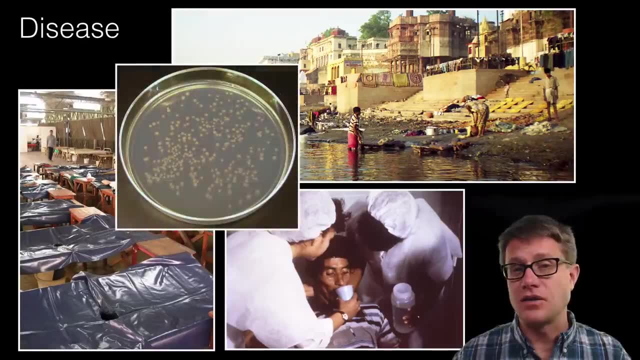 South America are awful, But it is a bacteria that is moving into the wastewater, and then we are drinking it back in, And so there are so many diseases that can be found in water, And so scientists use an indicator, species like E coli or fecal coliform numbers, And 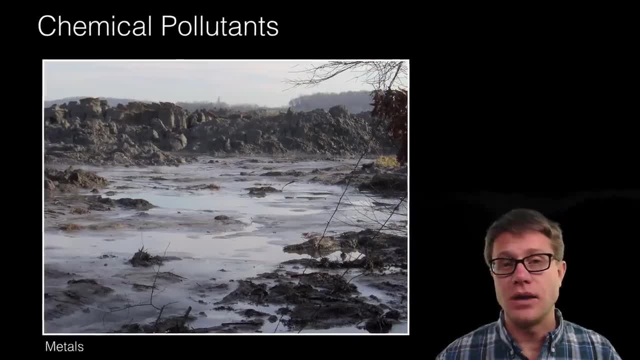 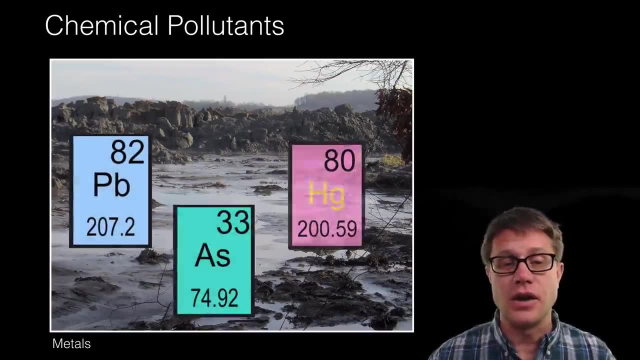 we can see. if that is found in the water, then we are going to find other diseases there as well. Now, aside from wastewater, we can have chemical pollutants. This is a big ash spill And we are moving a lot of chemicals into the water itself, like lead. 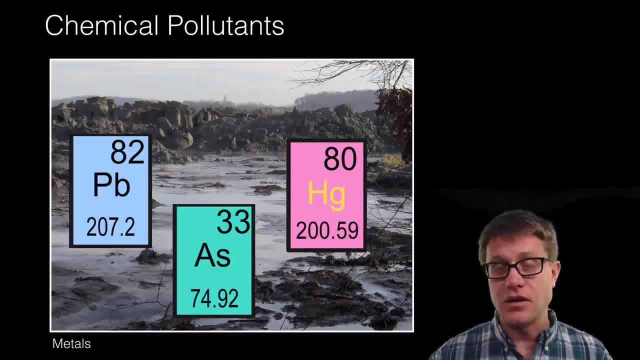 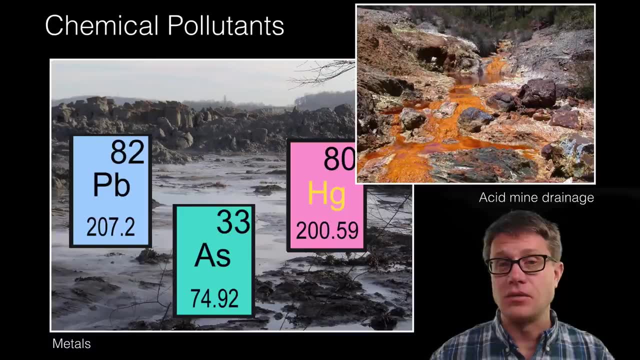 arsenic and mercury. Generally these things are going to be found underneath the earth, But with mining we are moving them up and they are getting into the water. We also have that same problem with acid. So acid mine drainage is being released, But it used to. 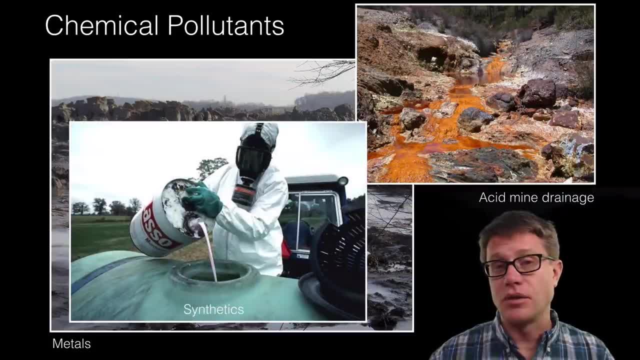 be trapped underneath the earth. We also have synthetics that we are producing, like pesticides, And then, finally, oil. We are pumping it underneath the earth, But now it can be found in the water, And so we are going to have a lot of things that are going to be found underneath. 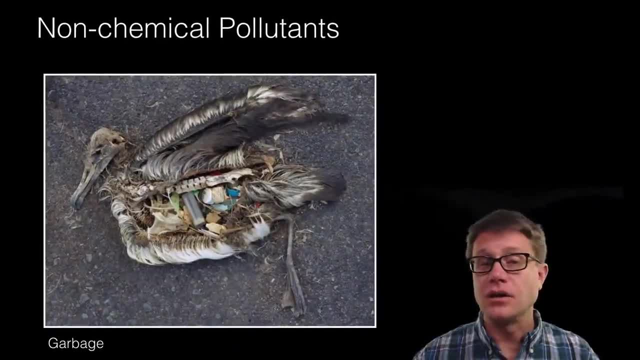 the earth. And then finally, oil. We are pumping it underneath the earth, But now it can be found in the water itself. And then, finally, an asteroid that was found on that, combined with an ash spill. We can also have non chemical pollutants, So this is a pretty sad picture. 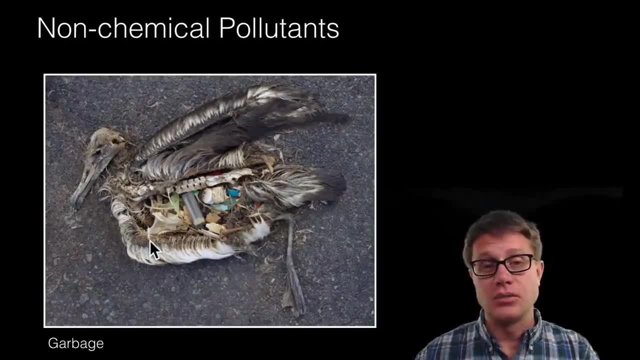 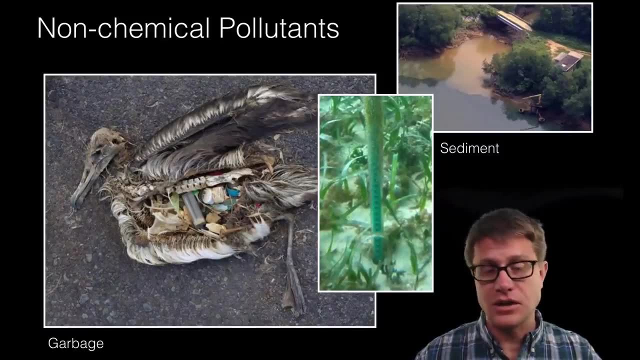 This is an albatross chick And its mother was feeding it And the father was feeding it- debris, marine debris. They just thought it was food And eventually the chicks are dying as a result of that, But it can also be sediment Dirt. So this is a construction zone And 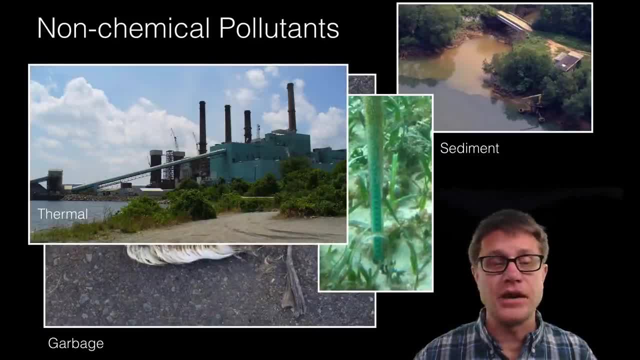 a lot of that dissolved sediment is moving into the water supply And then finally it can be heat, And so at this power plant, as a result of that combustion, we are moving a lot of that heat and electricity, And so we are going to than going to close this Youtuber thing off in history. 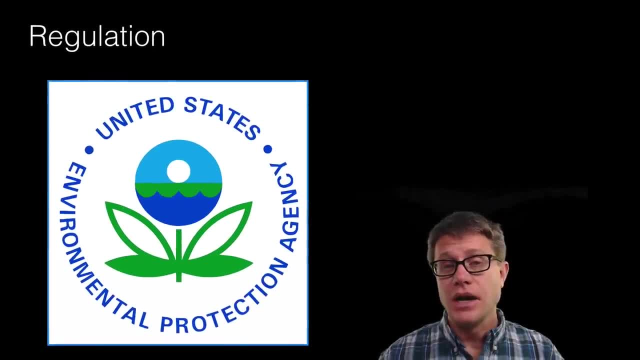 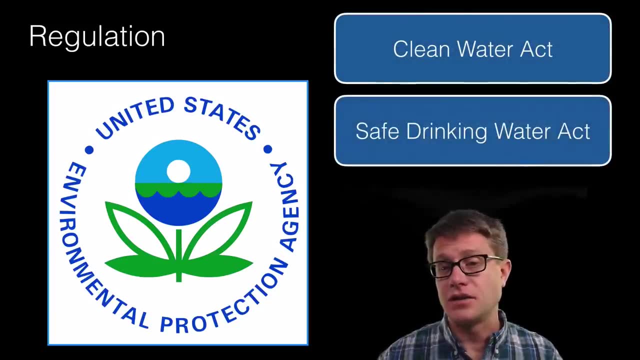 And then potato describes that other chemical activity. all the time that was going to happen 気, And that is impacting the environments as well, And so we have been regulating this since the 1970s, And so the most famous one is the Clean Water Act, But we also have the 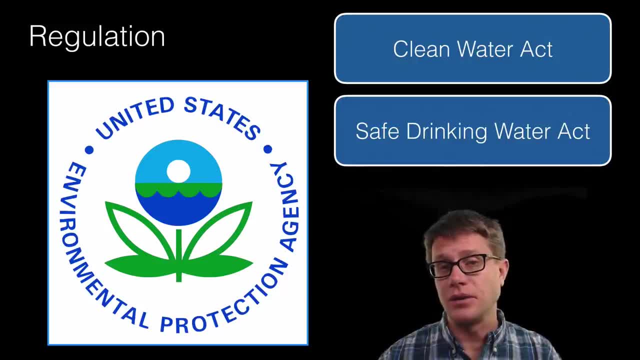 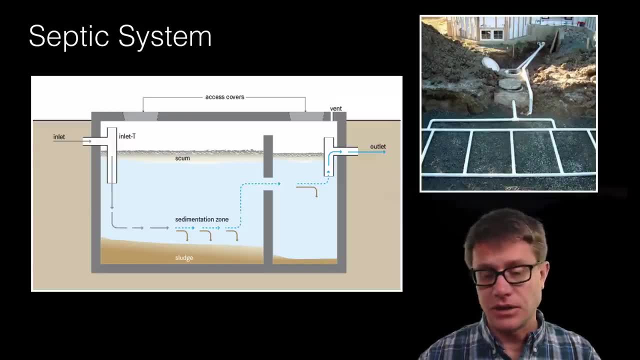 Safe Water Drinking Act. And what they do is they put regulations on the amount of pollutants that can be moved into the water supply Standards as far as water pollution. So how do we clean it up? We can use something like a septic system to treat our sewage. So the sewage 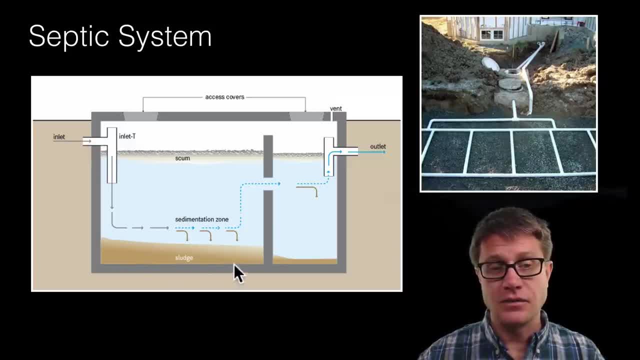 moves in here, Then you will get a lot of the sediment settle out And the scum will be on the surface, And then what you have is bacteria this whole way that are working on it, And so they are moving it out into a drain field And the bacteria are breaking. 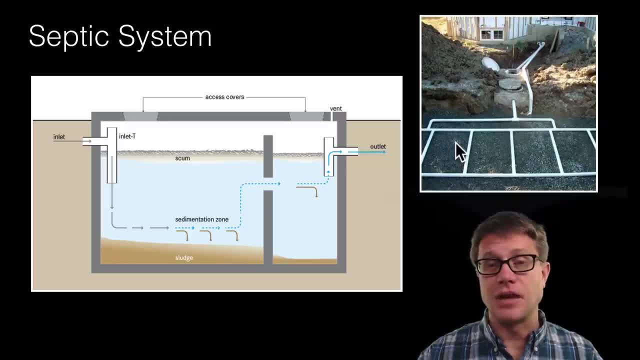 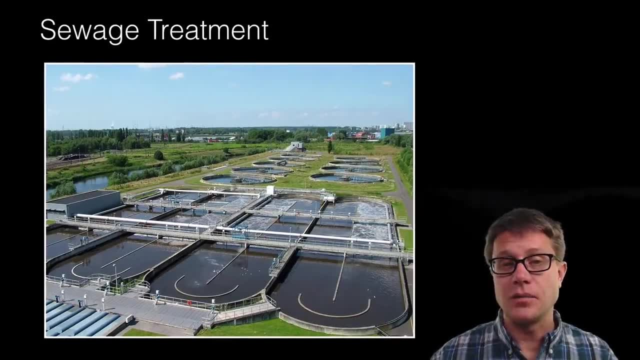 that down. Now the problem is if some of it gets out of the septic system or the septic system fills up, we can get leaching and it moves down into the ground water. This is a sewage treatment plant in Europe, And so the parts of sewage treatment are pretty simple. 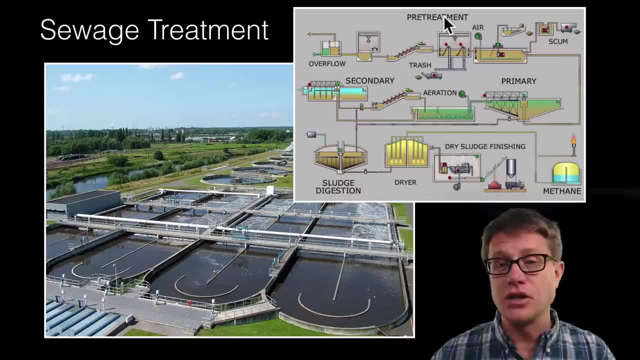 First of all, you will get pre-treatment, where we are moving things like big bits of garbage out of it And we are treating it with a little bit of oxygen. But then generally what we are doing is generally you have a primary treatment And so in this case, what you are 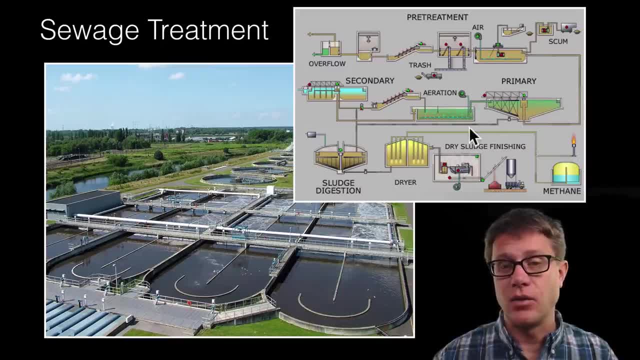 doing is you are letting a lot of that sediment settle out, And that is going to take one pathway where we digest it further, dry it out, And lots of times it moves to a landfill, But then we have these big tanks where we are aerating it. And so what you are doing 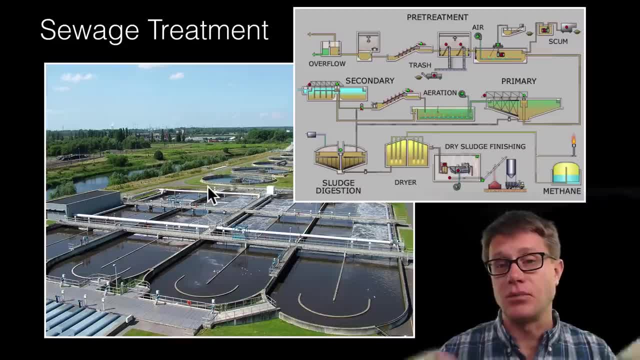 is bubbling oxygen into it, So these decomposing bacteria can break down that waste And eventually it is going to move into the water supply, Maybe back out into a river, once we have hit the right BOD level. After it comes into the river, then some of the sediment is going to come out of the